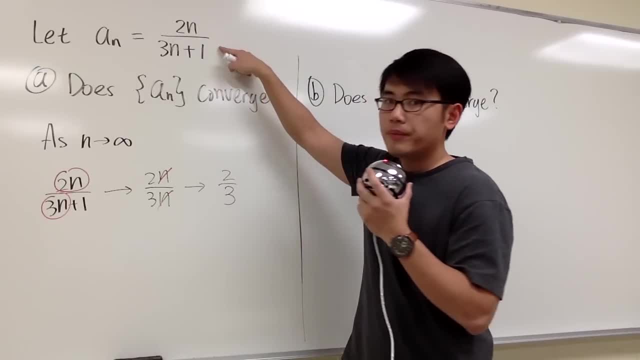 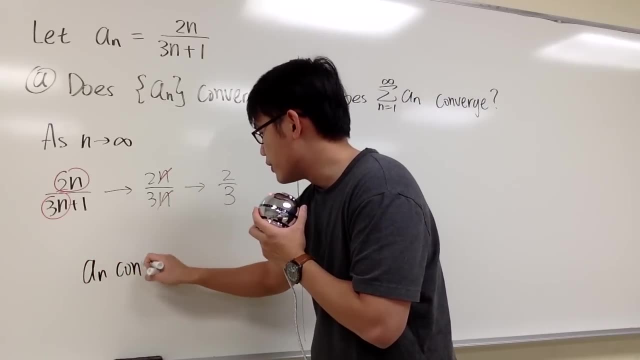 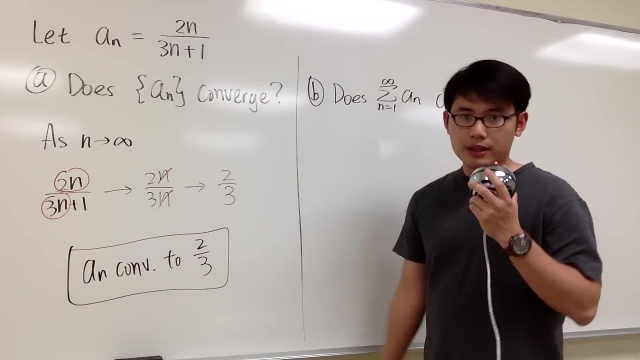 finite number. therefore, we know that this formula- right here the sequence converge- converges to 2 over 3.. So we can say a n converges to 2 over 3 and this, right here, will be the response. for that part, does the sequence converge? All we need to do is just take the limit. All right, let's look at. 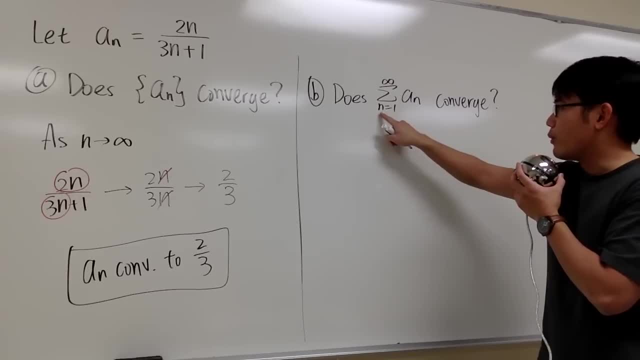 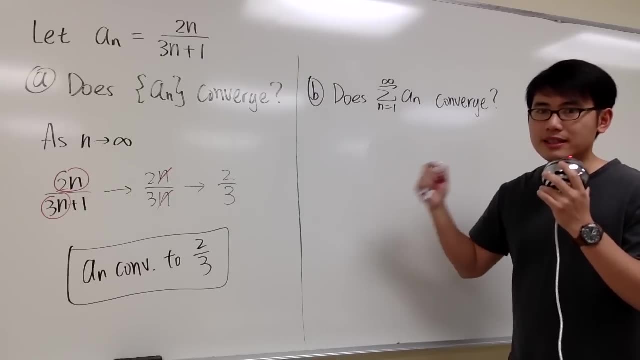 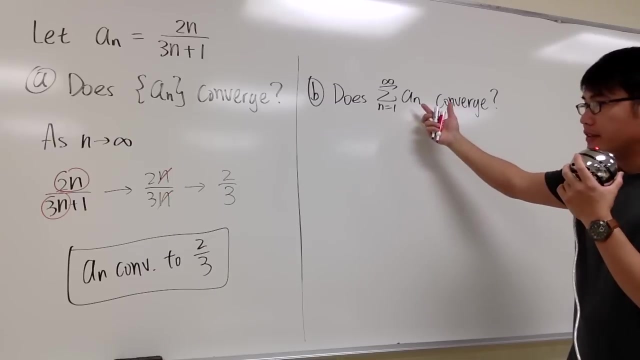 this one Does the series, the summation from 1 to infinity, a n converge. So the difference between a sequence and series is that a series it's a sum of bunch of numbers and those numbers are just a sequence. Okay, so we're talking about a n again, In another word. 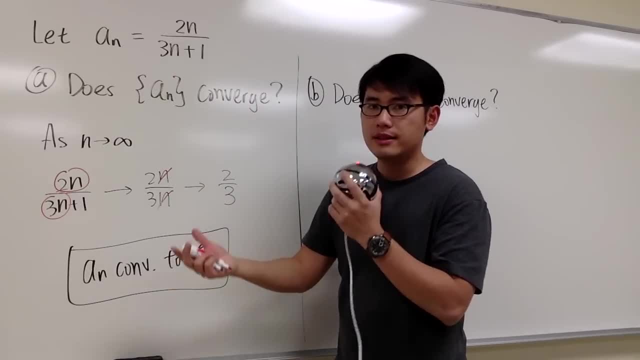 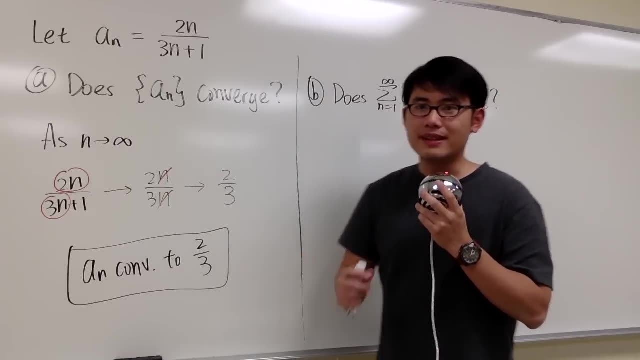 if you look at these values plugging, n is equal to 1, n is equal to 2, and they produce a bunch of values and then you're trying to add them up. Do we have a finite sum? That's what this question is asking us. Does the series converge? Do we get a finite sum? 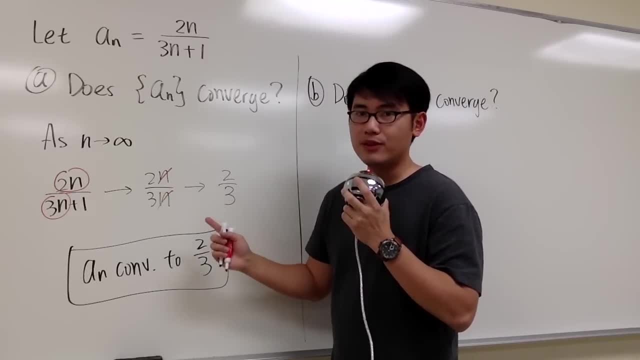 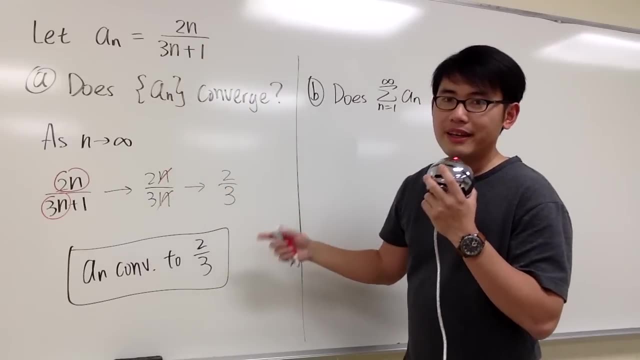 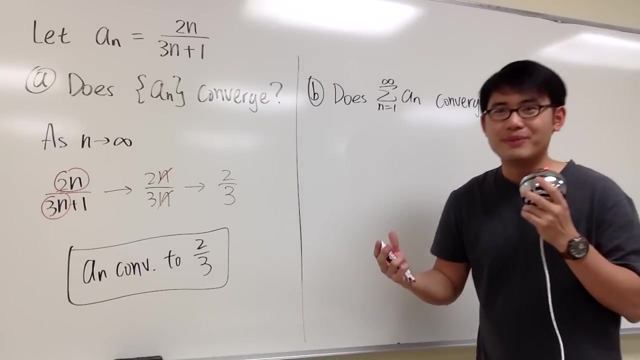 So one way to do it is: let's worry about what will happen eventually to this formula As n goes to infinity. we know that a n approach to two-thirds. In another word, eventually we pretty much just have two-thirds, two-thirds, two-thirds, a lot of them, infinitely many of them. 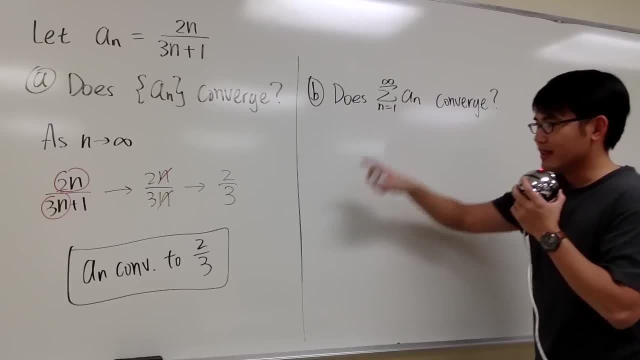 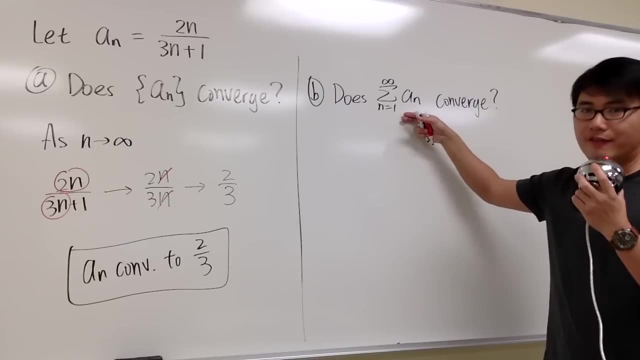 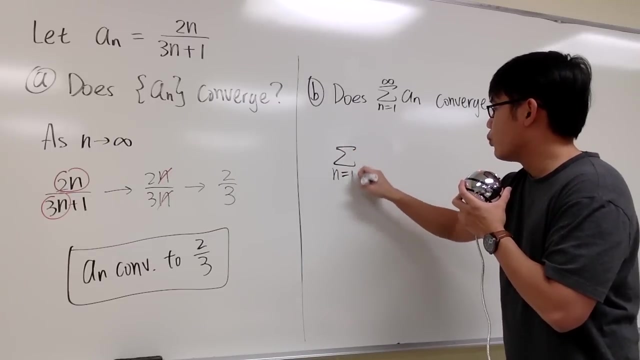 right. and if we add up a lot, a lot, a lot of two-thirds, what do we get for the sum? We will end up with positive infinity. Therefore this right here diverges because we do not get a finite sum. So we know that we can say the summation 1 to infinity: a: n. This right here is a. 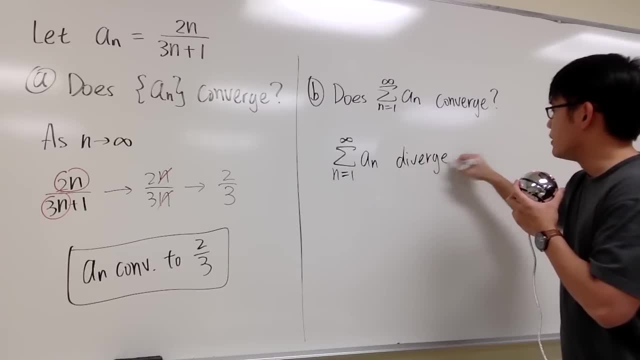 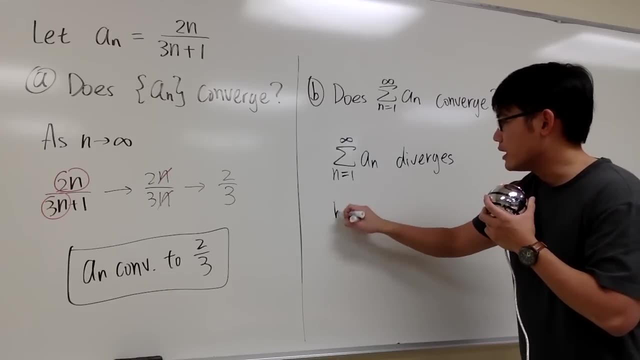 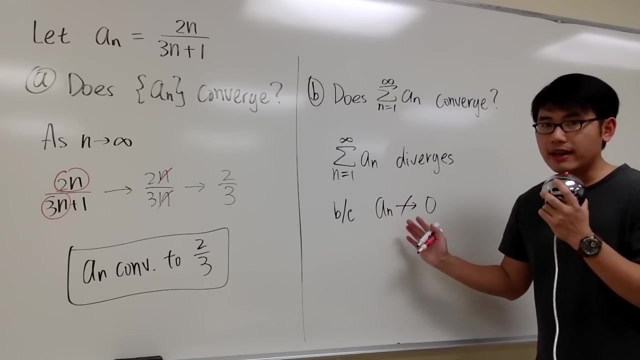 series. This right here diverges and we technically know that it diverges to positive infinity. but then we can just say it diverges and the reason for that is because we know that a- n does not approach to zero, because the only way that we can possibly have a finite sum is that this formula 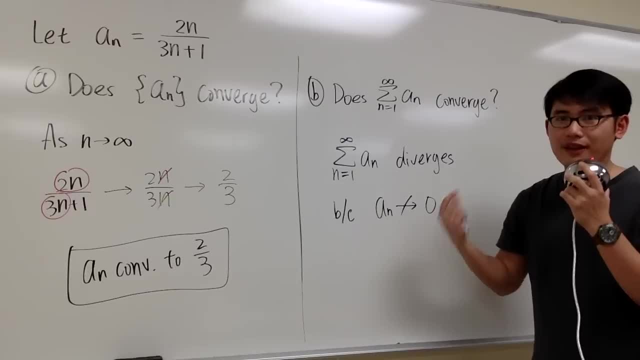 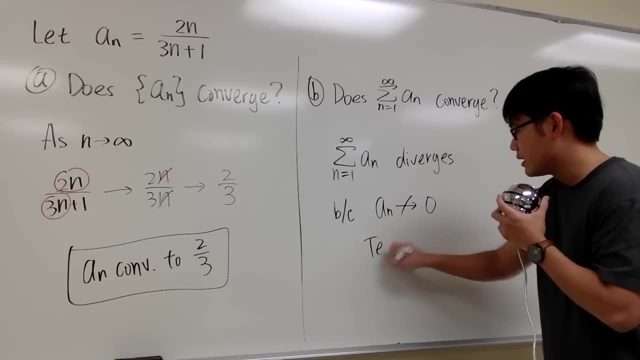 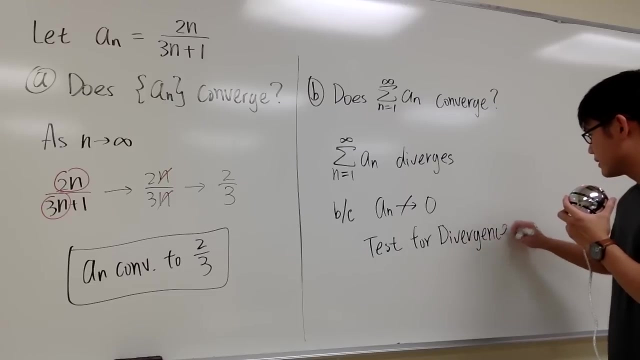 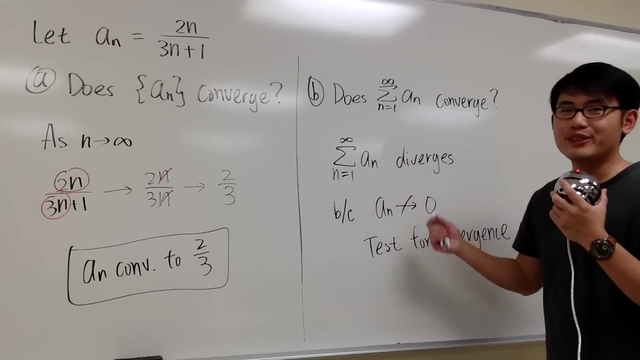 inside approach to zero and that's the test of divergence. so we can say this right here: because a n does not approach to zero and that's the test for divergence, and whenever this happens we can draw the conclusion right away: if a n does not approach to zero, we know the series diverges, so that's good.